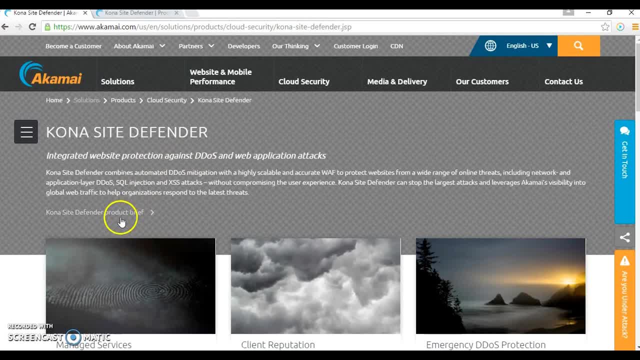 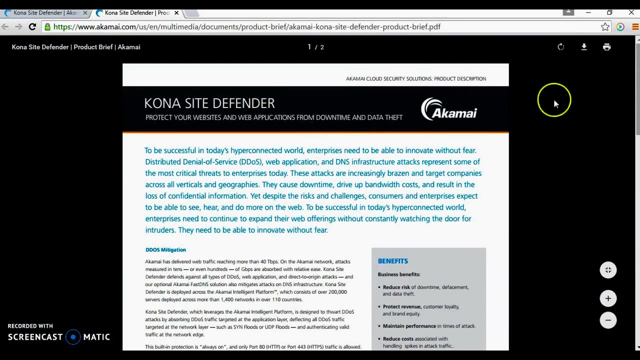 you can be on this page And then you go to Kona Site Defender product brief. So Akamai uses this suite, which is called KSD Kona Site Defender, to explain their WAF security solution. So I'll go through quickly this product document. 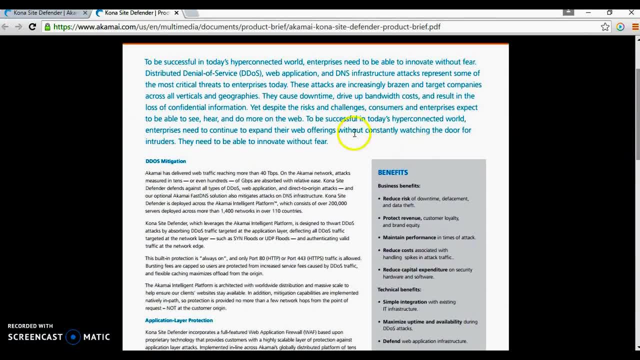 To start with, WAF is used for DDoS protection, which is shown here Recently. there is a high number of increase in DDoS attacks. So you can see that there is a high number of increase in DDoS attacks. So you can see that there is a high number of increase in DDoS attacks. 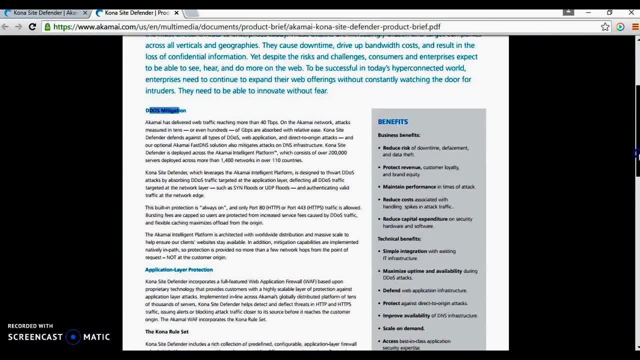 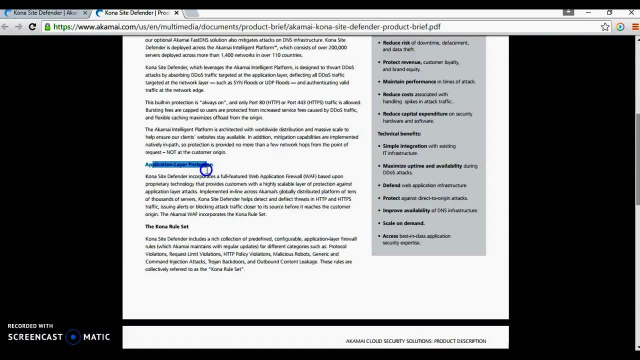 So you can see that there is a high number of increase in DDoS attacks. So WAF helps to protect from that. How does it protect it? It's listed here, starting with application layer protection. So WAF have a component called Kona ruleset which is used to design the rules. 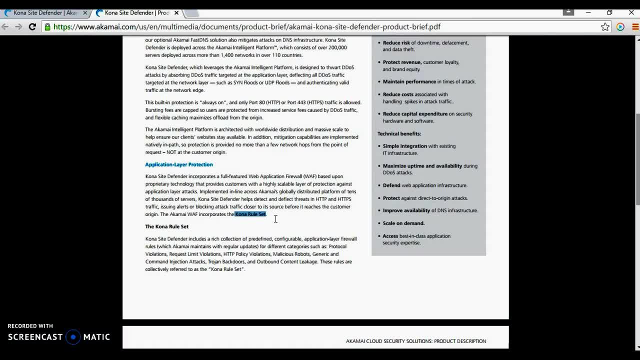 It's pretty much similar to IDEA signatures and these ruleset whose come from OWASP CRS. You can research about CRS rule sets separately, but these rule sets are designed by Akamai engineers for different attacks on the well application. okay, and these rule sets can. 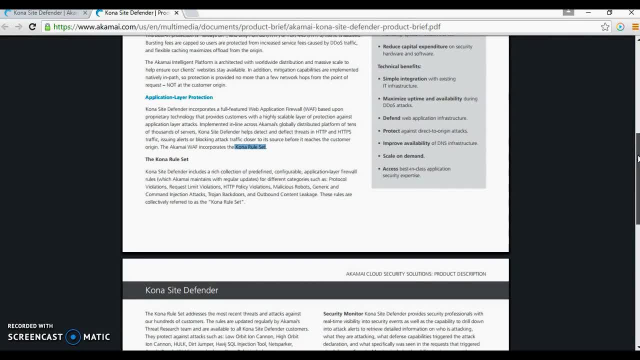 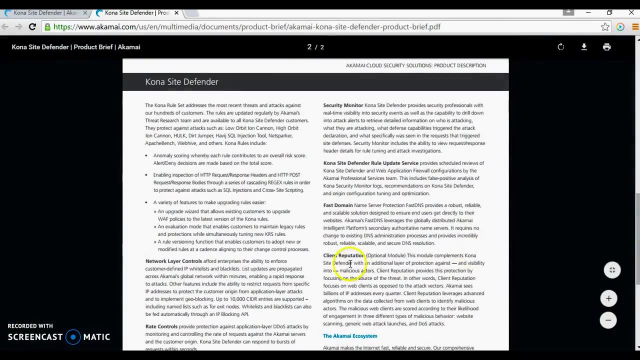 be turned on for alerts or for deny, so you can decide if you want to put a rule in alert mode or deny mode, because if an alert mode will just send you an email but if it's in deny mode then it will drop that traffic, okay. second component: 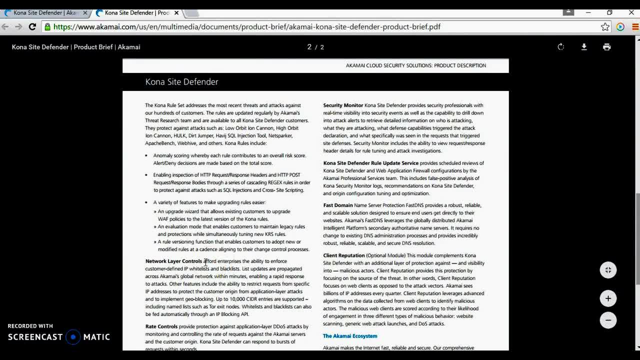 is network layer controls. this is about the old-school. so whitelisting and blacklisting. so you can either whitelist your IP addresses, your client's IP addresses, who you want to connect to you, or you can blacklist the attackers IP addresses. this also gives you an option to whitelist some IP addresses because 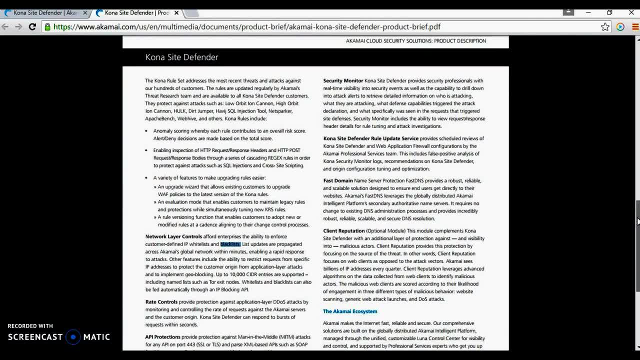 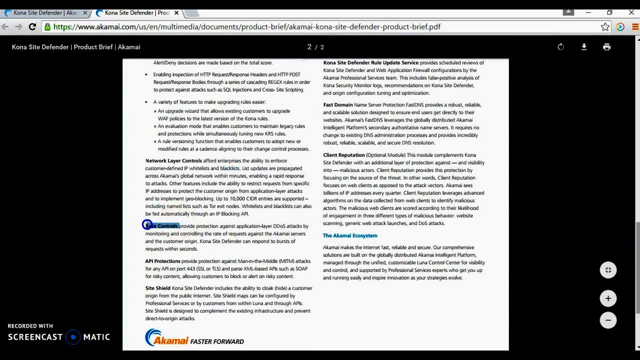 you could be hiding some IP addresses from your client, or you could be hiding some vulnerability testing going on in your company and you don't want to generate alerts or deny that traffic, so you can just bypass those IP addresses. so that's also an option. going to the next one, which is about rate controls, so 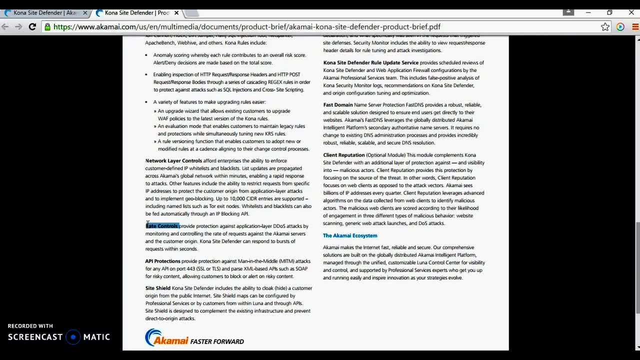 rate controls are for volumetric attacks and that could be like an attacker trying to bend on your website by generating 100 attempts per second or in less than five seconds. so you can put a threshold for your rate controls and stop those volumetric attacks. next one I'll cover is side shield, which is about 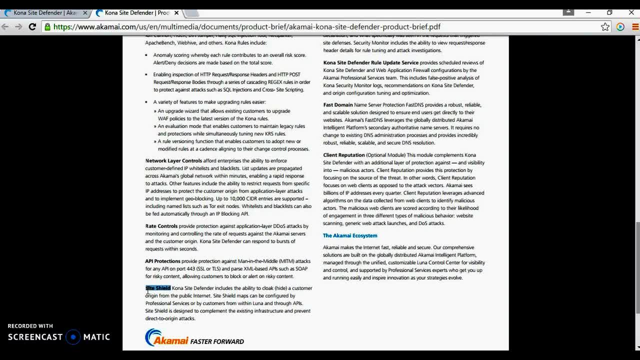 protecting your origin so that the attacker or the outside world doesn't know the IP address of your web server. so Akamai will do the DNS part for your web origin server and replace the IP address. so the attacker or the client will only see Akamai's IP address or any other IP address. 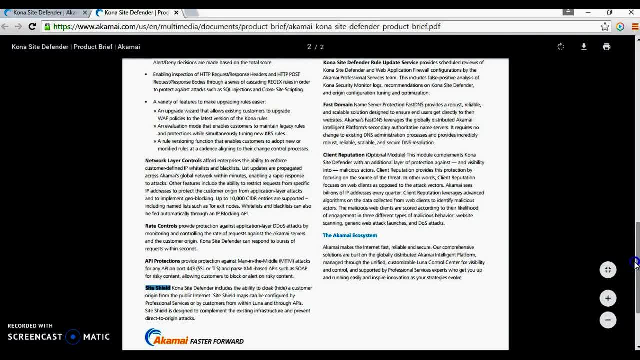 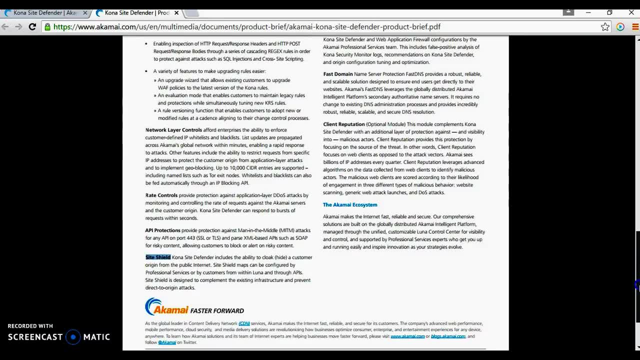 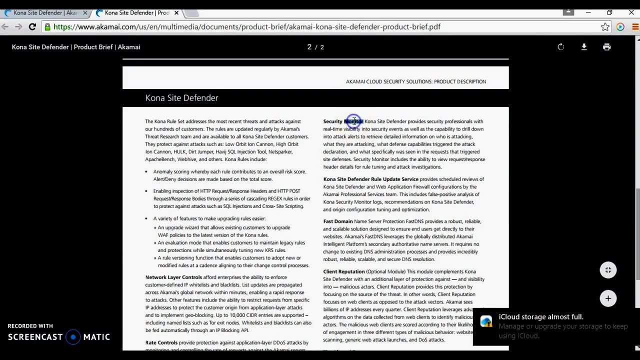 application, firewalls, vendors, IP address- instead of exposing your IP address, which is a side shield, putting a site in front of your origin server security monitor. this is about monitoring the attacks. so this has a nice dashboard which generates alerts and you can tune down what kind of alerts or emails you. 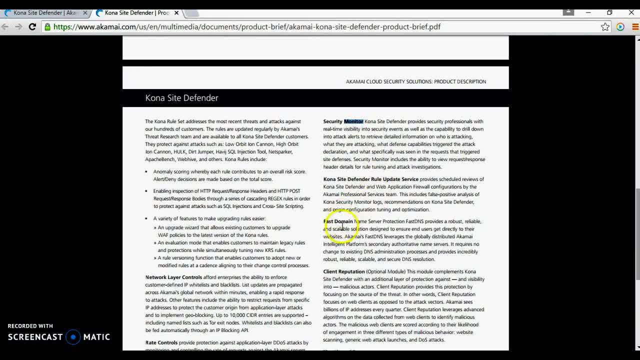 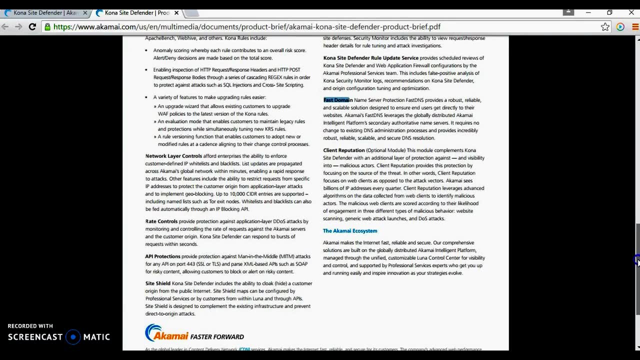 want to get. so that's monitoring part for these alerts. and then the other components are minor components I won't be covering here, but fast DNS, for example, is for the DNS changes and similarly other components. so that was a small introduction about Vaf and particularly Akamai Vaf. thanks for watching. 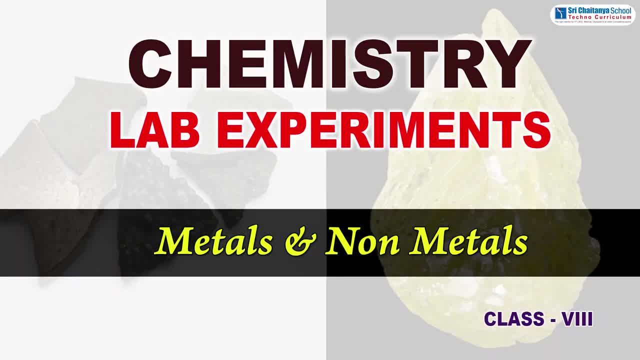 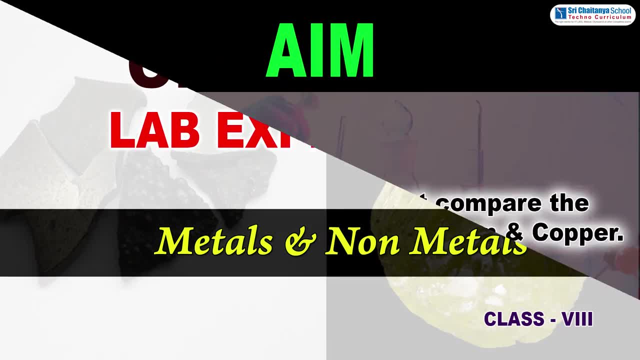 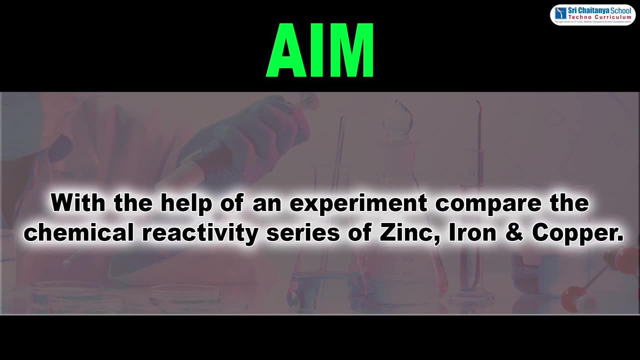 Hi students, today we are going to do an experiment based on the chapter metals and nonmetals for class 8th standard. The aim of this experiment is, with the help of an experiment, compare the chemical reactivity series of zinc, iron and copper. The materials required are: